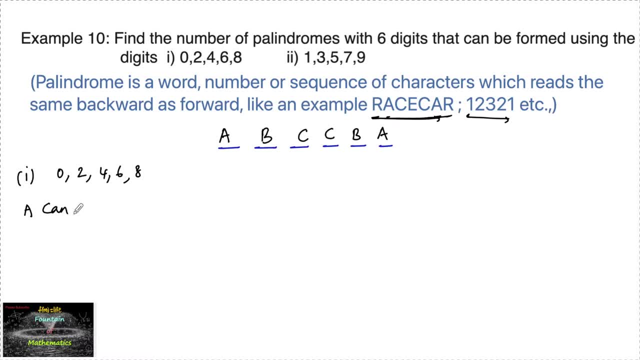 first place. So now A can be filled. A can be filled in where 0 cannot be taken. So how many possibilities are there remaining? 2, 4, 6, 8.. So A can be taken either 2 or 4 or 6 or 8. So we can. 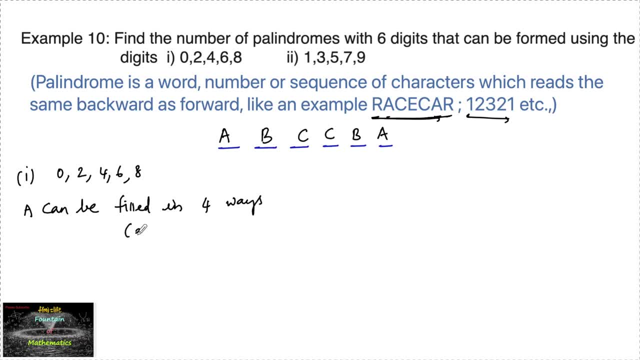 A can be filled in four ways, excluding 0.. And now B, the second position. B can be filled in. Now B can be taken any of either. 0 also can be chosen, So B can be filled among the five digits. Here the repetition is allowed, because there is no. 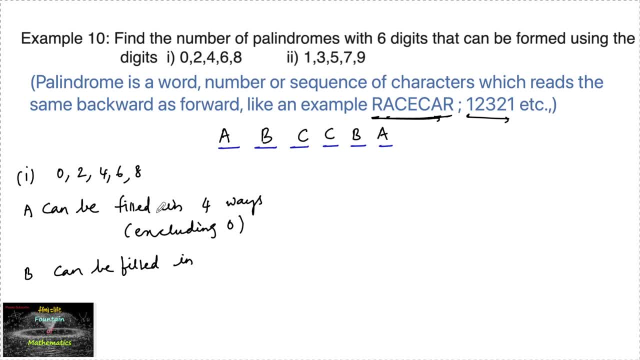 condition that we cannot repeat the digits. So repetition can be taken. So once digit is already fixed in the first place can be taken again. If suppose A is equal to 6 can be considered in the second place, also Because the digits can be repeated. 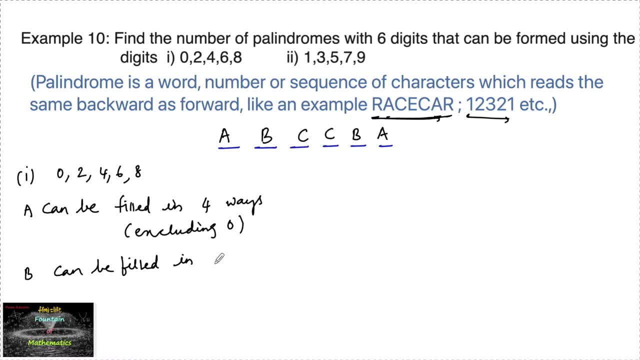 B can be filled in total five ways, including zero, So we can say including 0.. And now C. third place, C can be filled in again. see, also can be placed as 0.. 0 can be placed and 2 or 2 or 4 or 6 or 8 or anything. 0 can be placed, and 2 or 2 or 4 or 6 or 8, anything. If suppose B filled in equal 5 ways, This can be done, So we would be able to filled in all of them individually, so that C is considered in the button 1 and 6 place. Now B should be we there every four places. totaI make sure that writ a third place, C can be filled in only one place. Again, C can be filled in the place here, So we should be there anywhere. So let us check for any number of countries. 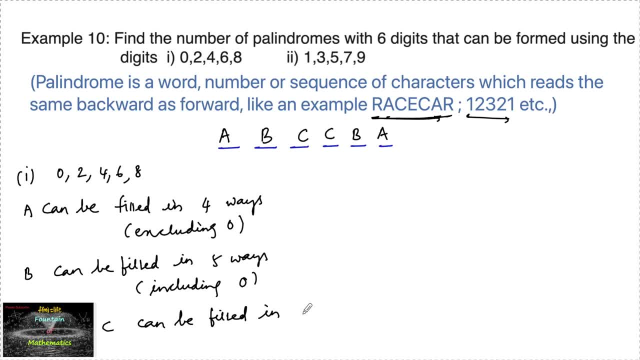 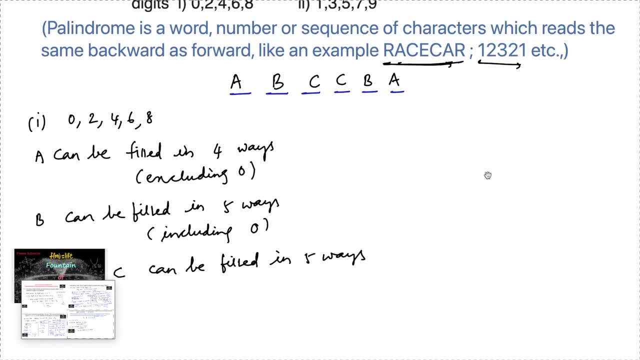 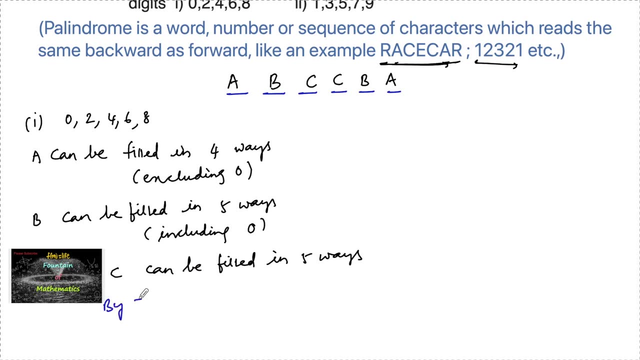 or six or eight, anything can be placed. the digits can be repeated also, so c also can be filled in five ways, including zero. so therefore we can say by multiplication principle, by fpc, we can say number of palindromes, number of palindromes by using the digits zero to four. six, eight is nothing but four into five, into.